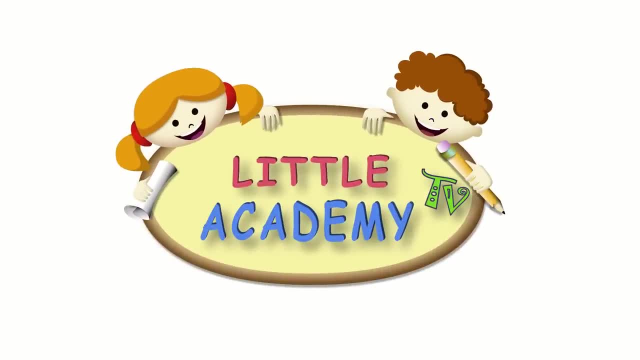 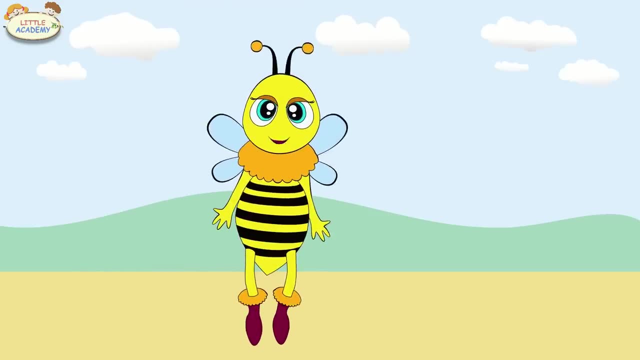 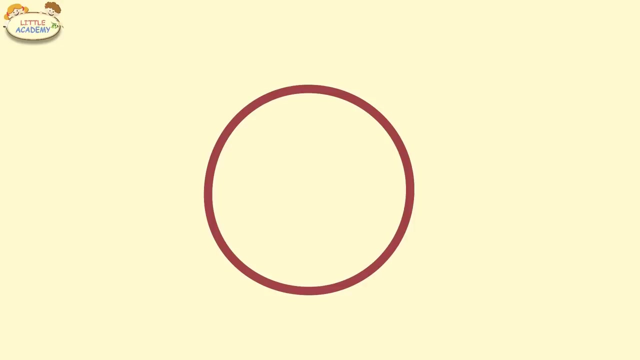 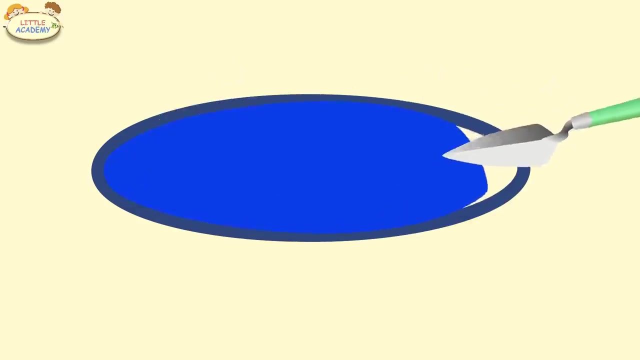 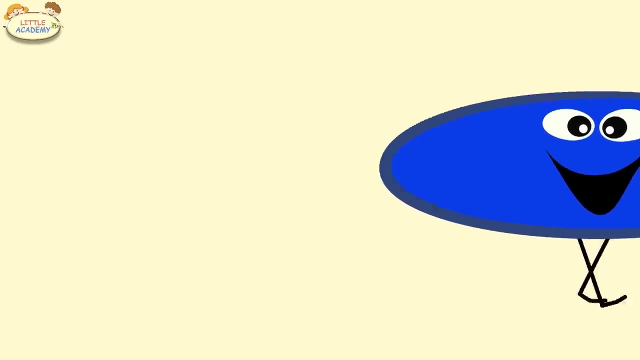 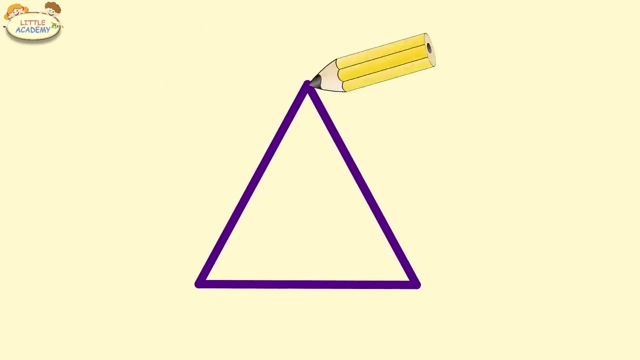 Hello again, I am Polly the bee. How about learning shapes together? Let's go: red circle circle. orange circle circle circle, yellow circle oval. green circle, green oval, oval, light blue oval. light blue, oval, oval, blue, oval, light blue, oval. triangle, triangle, triangle, triangle, triangle. 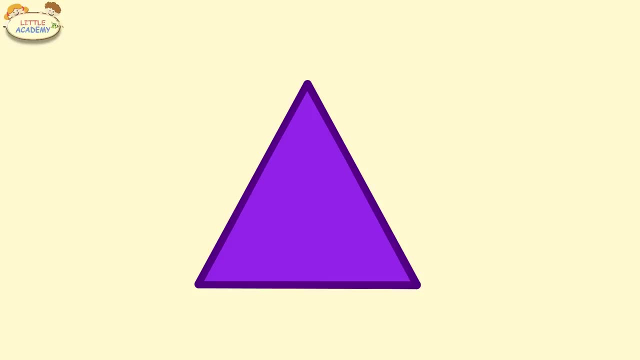 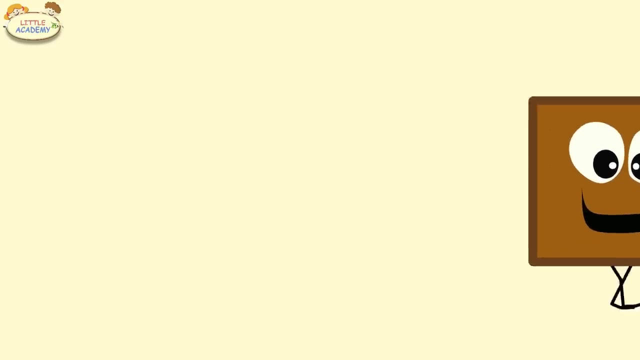 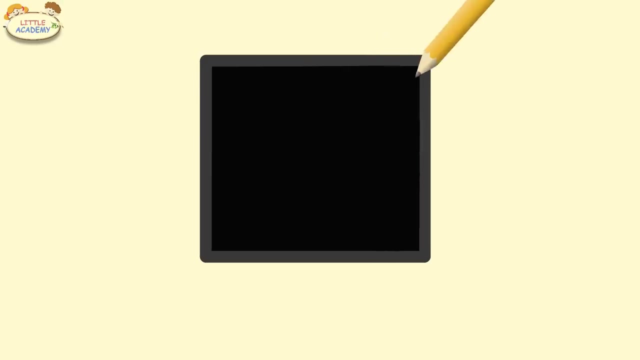 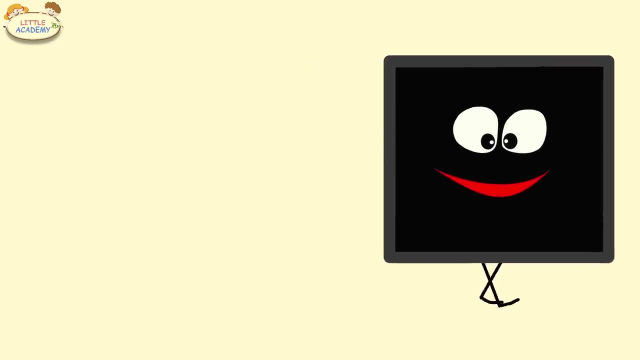 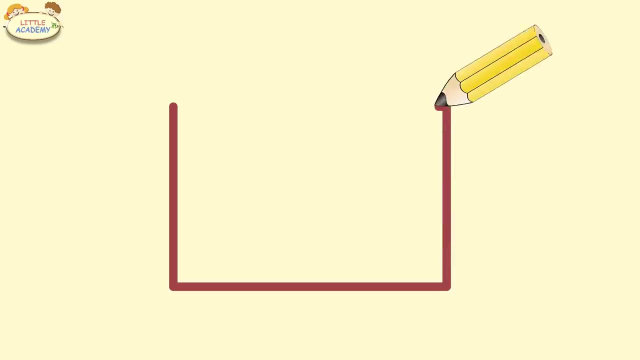 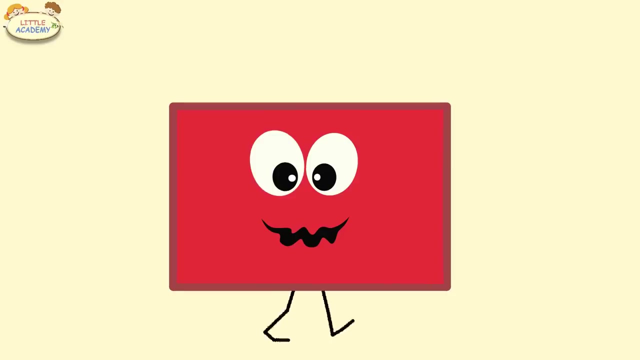 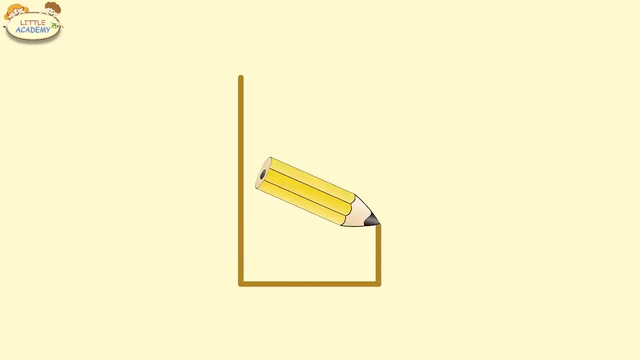 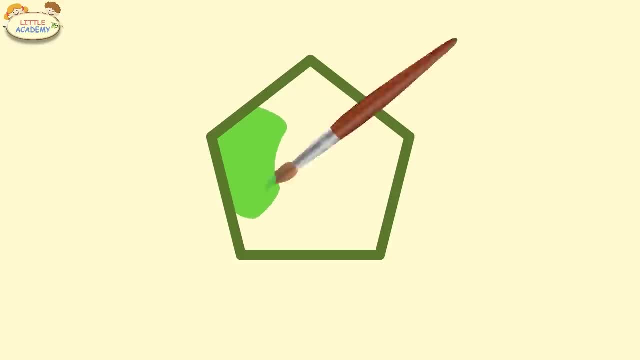 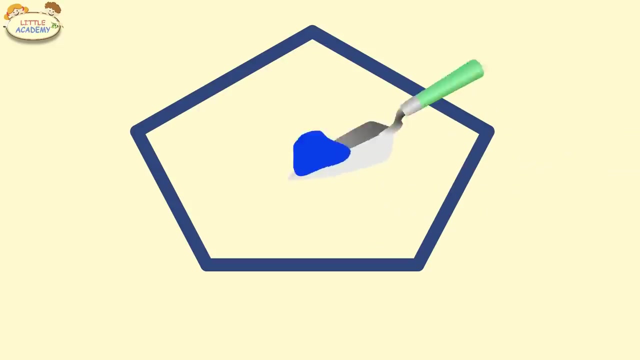 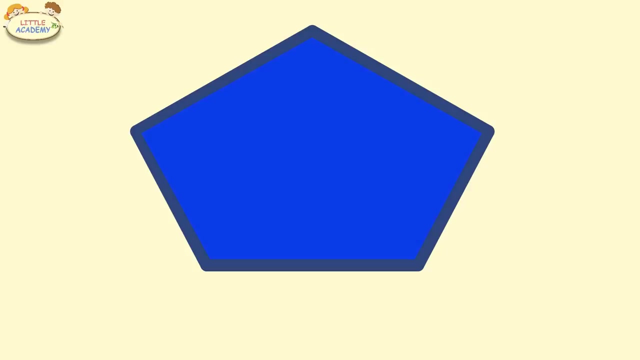 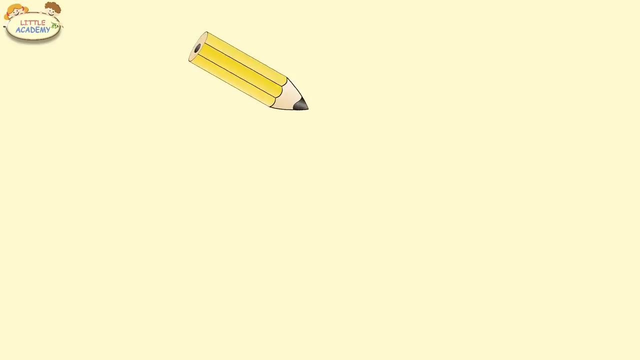 pentagon green- pentagon blue. pentagon blue- pentagon. pentagon light blue. pentagon. pentagon blue- pentagon blue- pentagon. hexagon purple- hexagon. Hexagon White- hexagon. Hexagon Pink. hexagon. Octagon Brown- octagon. Octagon Grey- octagon Grey- octagon. 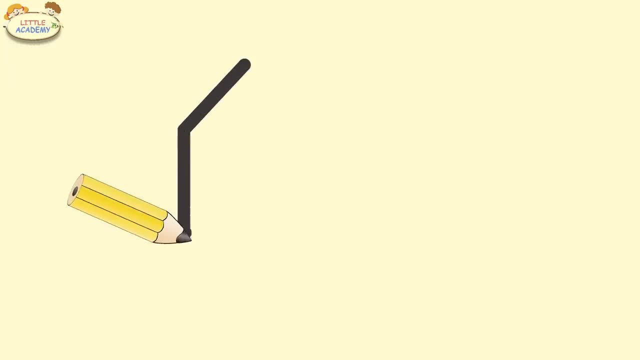 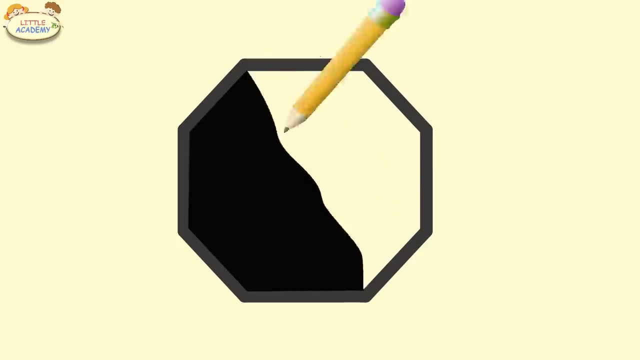 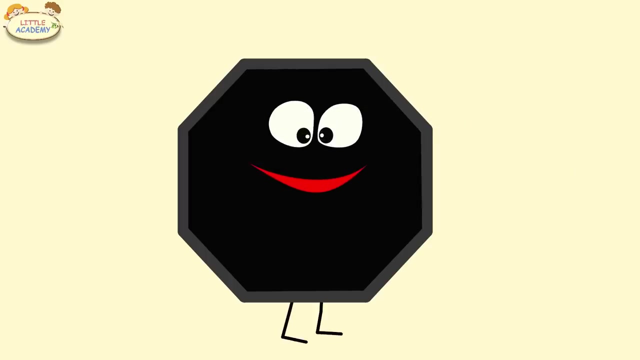 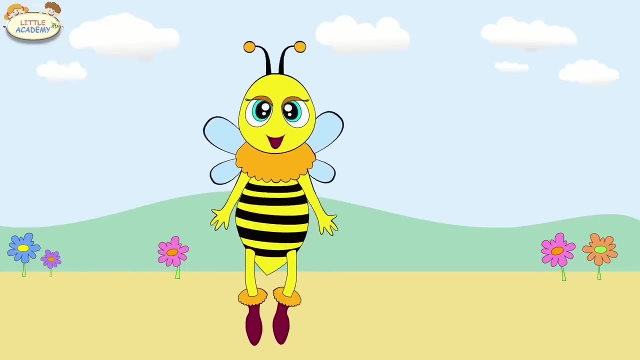 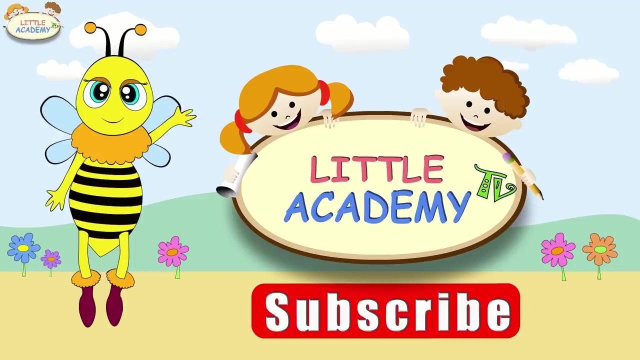 Octagon: Octagon, Black octagon. Great job, Subscribe to our channel and see you soon, Bye-bye. Thanks for watching.